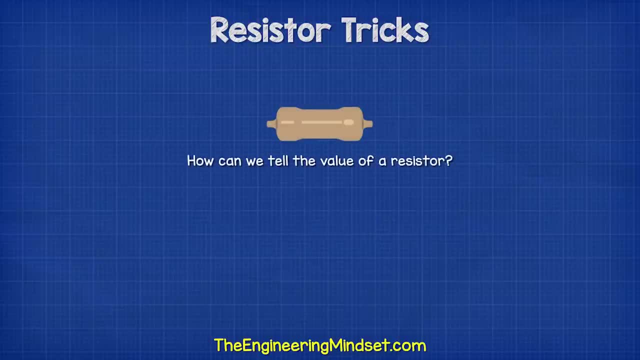 How can we tell the value of a resistor? Well, these coloured stripes on the body will tell us the value, but we will need to look it up on a chart. We can get four or five band resistors typically, So let's look at some examples of these, With the four stripe type. 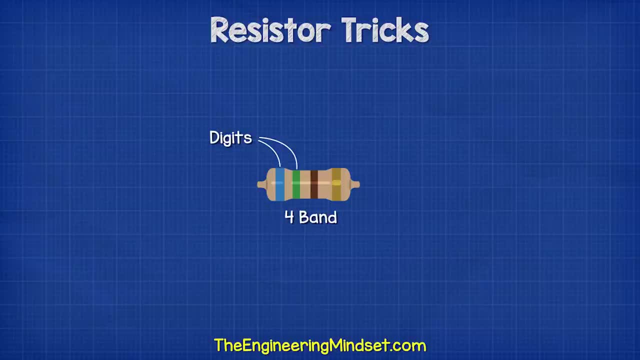 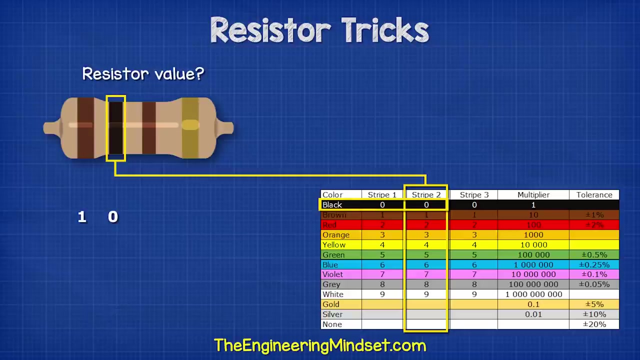 the first two stripes are the digits which we combine. The third stripe is the multiplier and the fourth stripe is the tolerance. For example, this four band resistor is brown, black, brown and gold. Band 1 is equal to 1.. Band 2 is equal to 0, giving us 10.. Band 3 is the 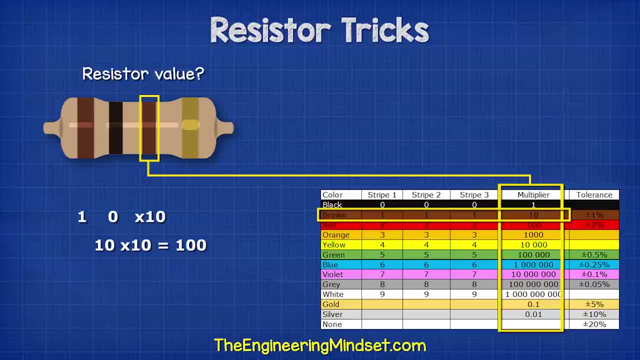 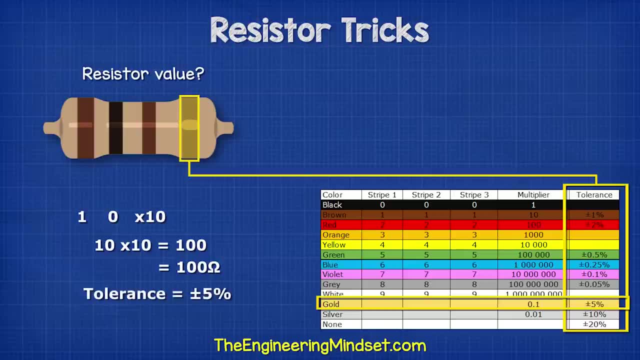 multiplier, which is 10.. Band 4 is equal to 0, giving us 10.. Band 5 is equal to 0, giving us 10.. So 10 x 10 is 100 ohms. Then the gold is the tolerance of 5%. So it could be as low as 95 ohms. 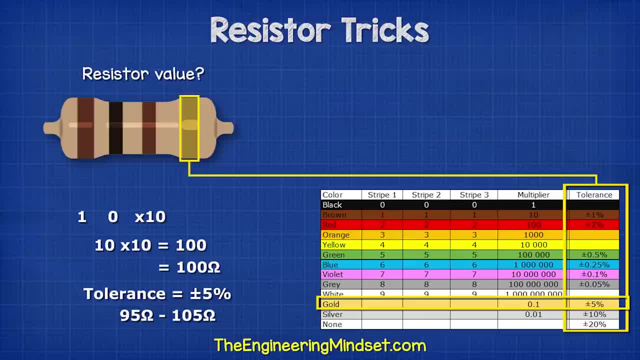 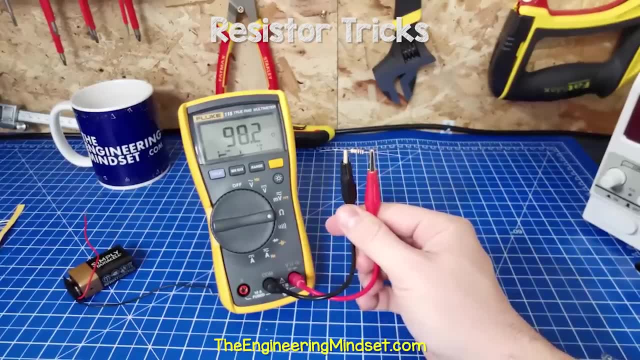 or it could be as high as 105 ohms. When I measured this one with a multimeter, we can see it was reading 98.2 ohms, which is within the tolerance. So we saw that the previous resistor wasn't very precise. If we need more precision, then we will need to use a different. band resistor to measure the resistance. For example, if I had a larger música resistor and these two cap will give us 0.5 ohms. The multimeter value I have here will be 0.5 ohms If I had 20 ohms. I will need to memotor it by paper. just in the second frame I see compound count. will I use a senate here to complete myuity? This will give us a total of 0.5 ohms and no data comes up out of it. 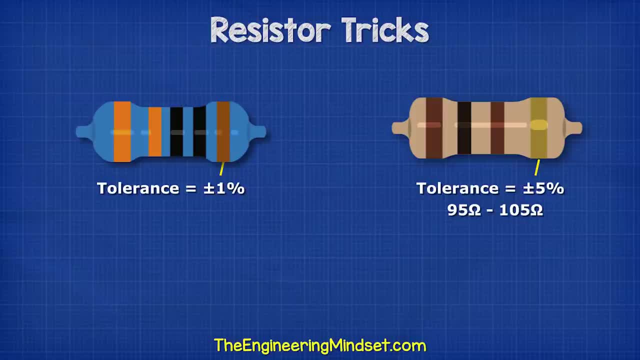 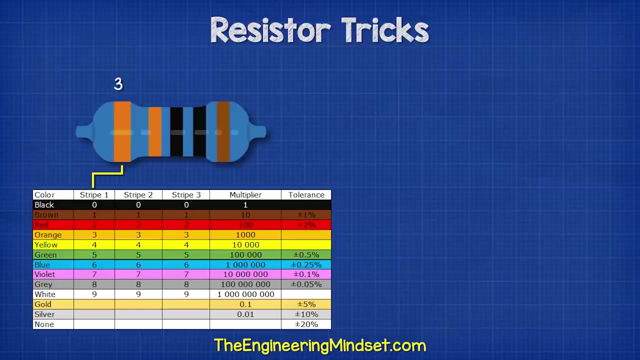 a smaller tolerance, like this: 1% tolerance, five band type. With this type, the first three stripes are digits, the fourth is the multiplier, the fifth is the tolerance. This one is orange, orange, black, black, brown. So this is a three, this is a three, this is a zero, with a multiplier of one, giving us 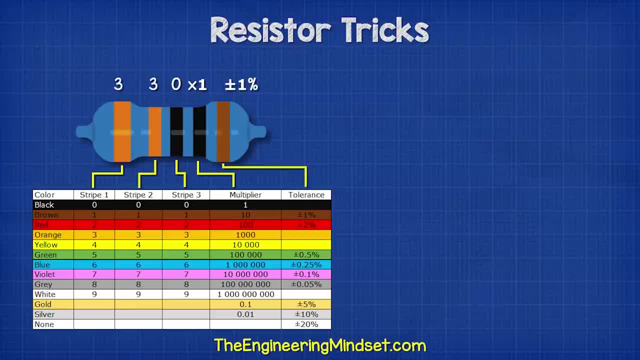 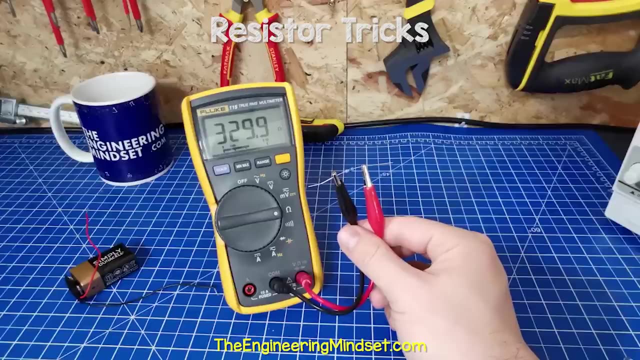 just 330 ohms. The tolerance is one percent, so it could be between 327 ohms and 333 ohms, but when I measured this one with a multimeter, we can see it was reading 329.9 ohms. so it's perfect. Okay, that's.